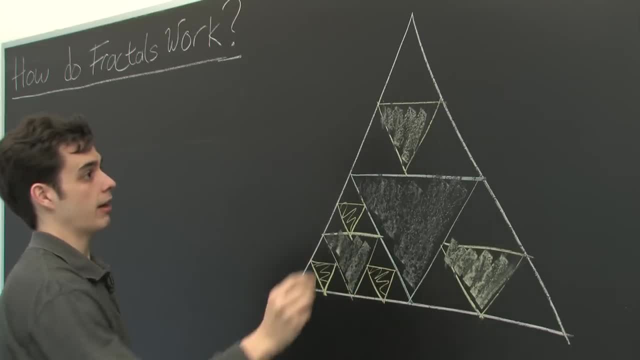 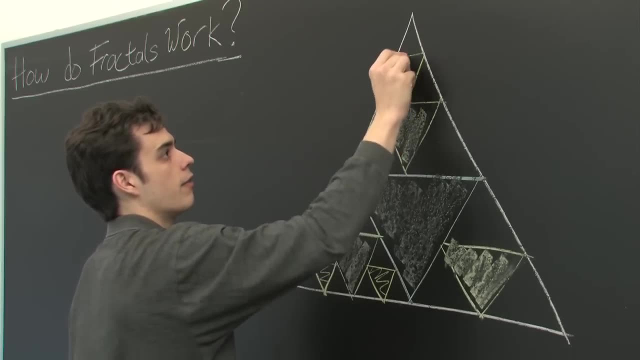 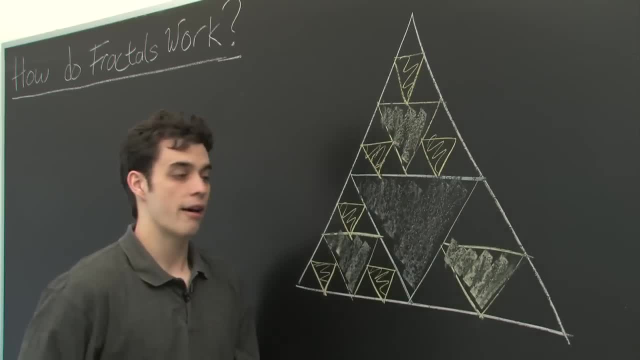 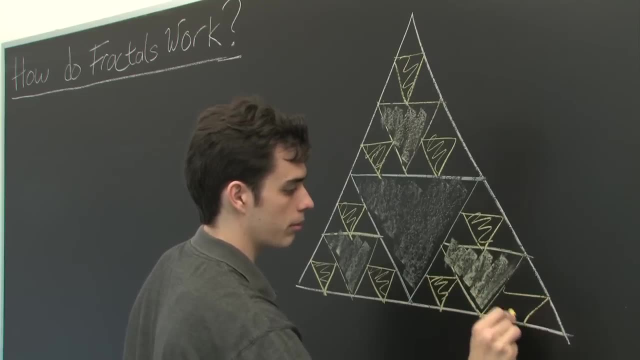 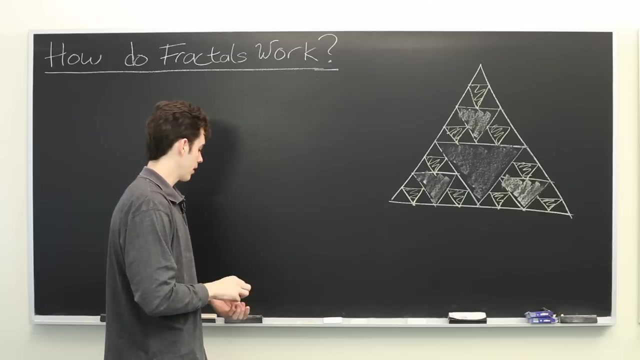 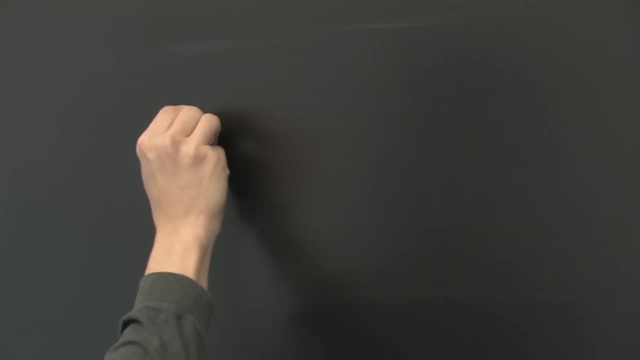 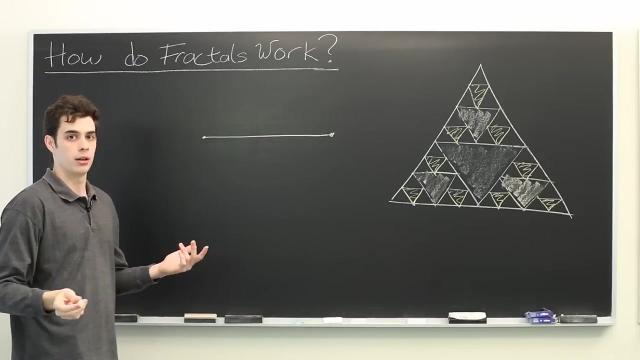 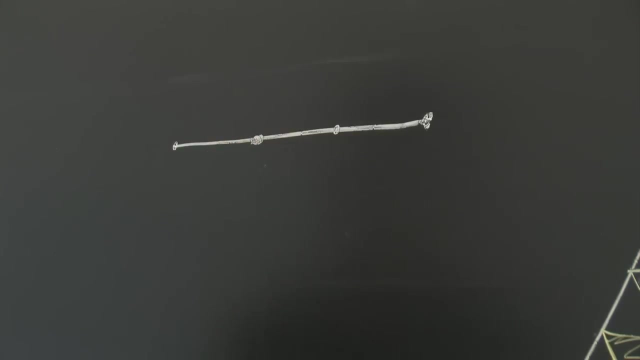 triangles. Now we're adding a total of nine yellow triangles, And so on and so forth. But there are many other ways to construct fractals. Another fun example is: Suppose you just start with something as simple as a line segment And from here we divide the line segment into three chunks, each of equal length. 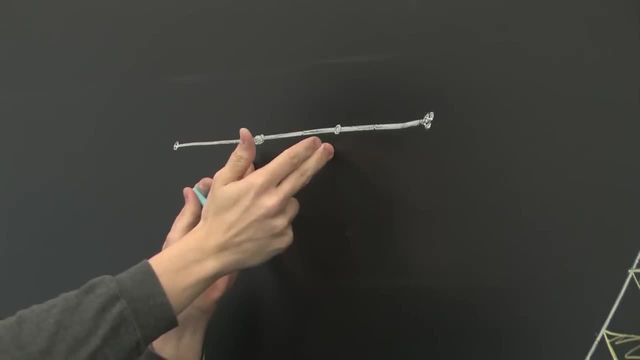 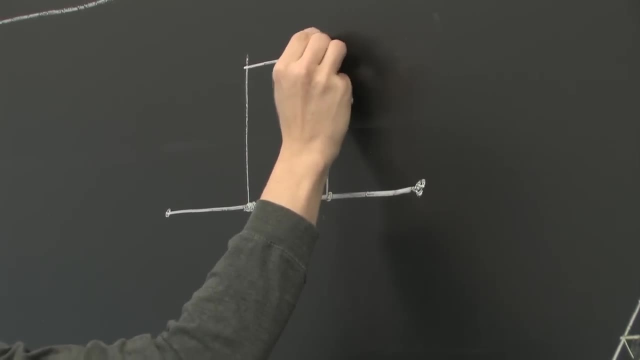 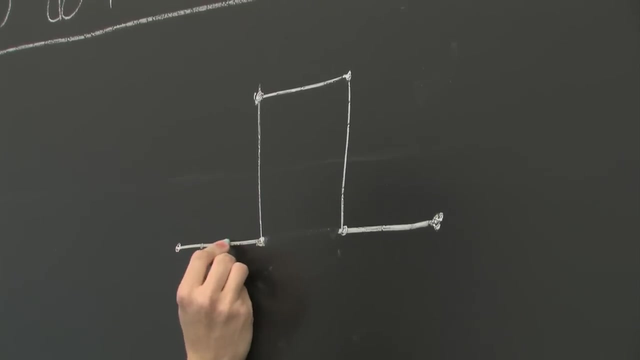 Then the first stage: we take the middle chunk of each line segment and make it into a square. Then we'll erase that middle segment. Well, let's repeat the process. So now we'll divide this into thirds, this into thirds, this into thirds, and so on. 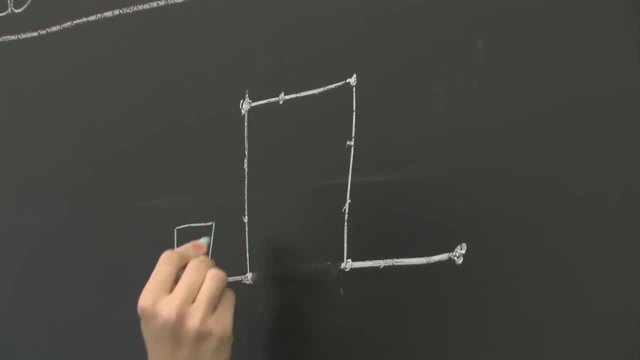 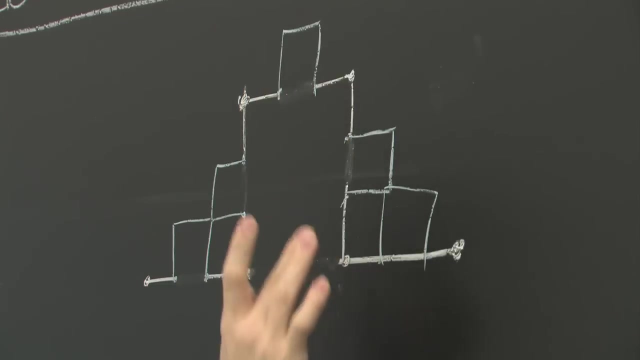 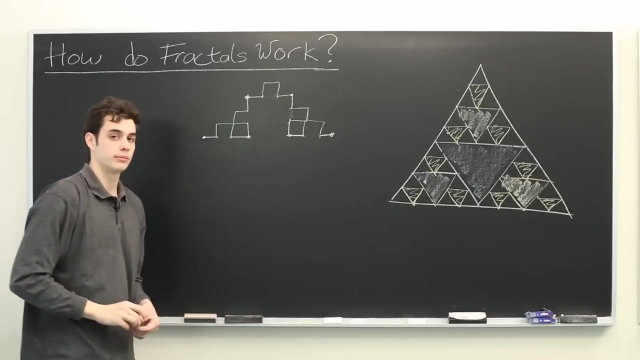 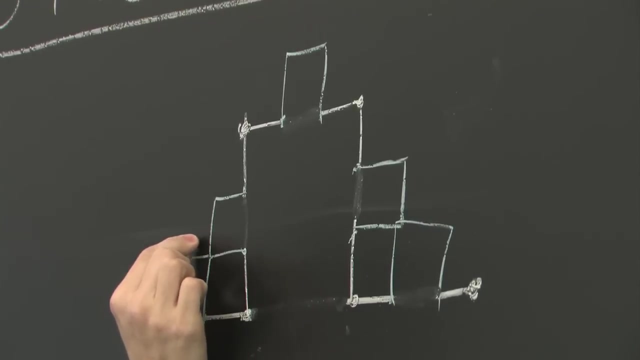 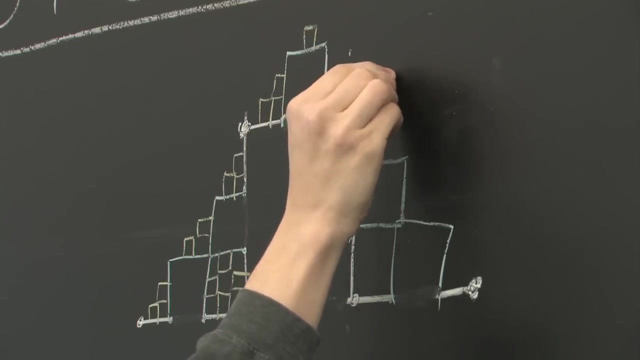 Make a square. make a square, square, Okay, Square, square. and then erase those thirds that we started with. Okay, Now let's repeat the process again, Start with here: draw a square, each of these, And so on and so forth. 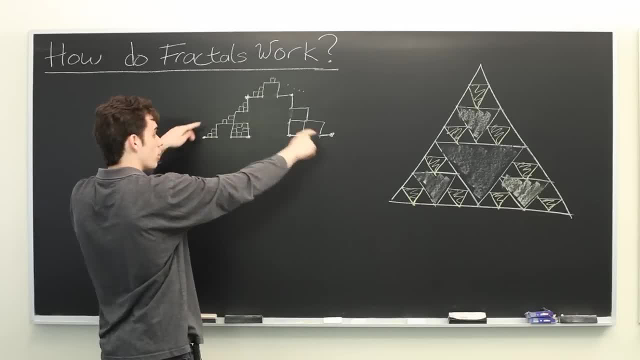 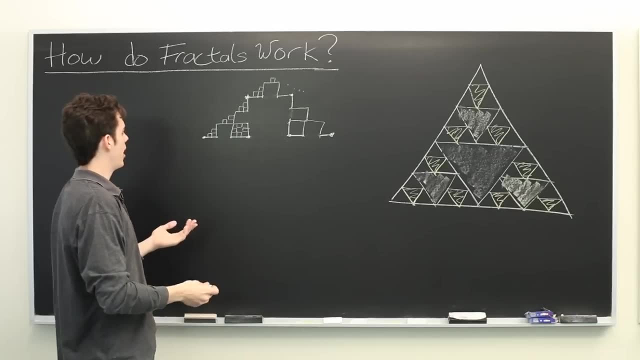 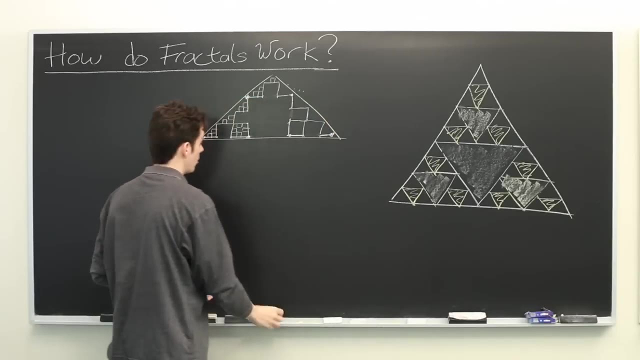 See that eventually, if you line up these corners, it'll start to look like a triangle, which is unusual. You think that, well, you start with a line and you start adding squares and the result is something that looks triangular. 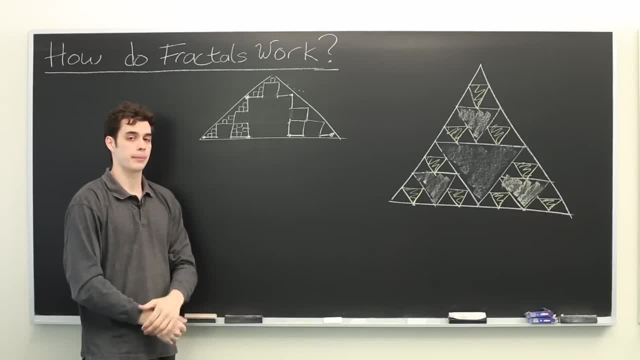 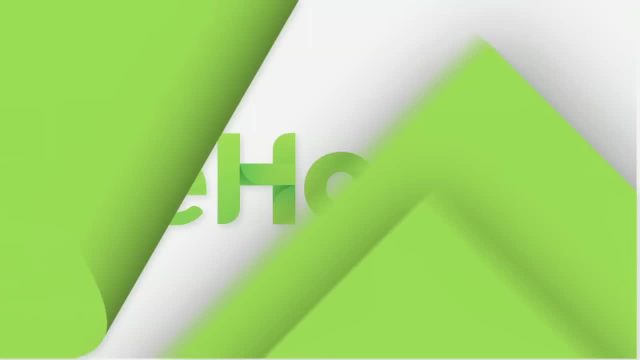 And there are many other ways that one can construct fractals. My name is Ryan Molloy and we've just discussed how do fractals work.